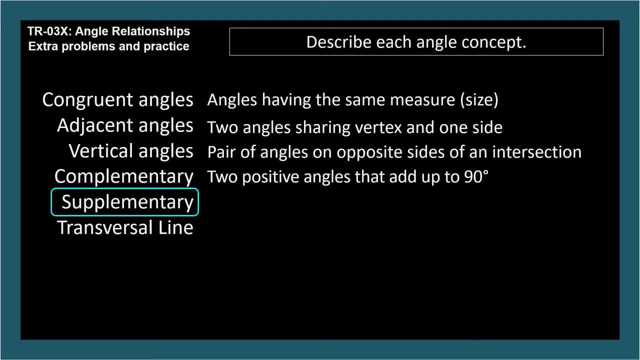 Supplementary: Two positive angles that add up to 180 degrees. Subliminary: Two positive angles that add up to 180 degrees. Transverse line Line that crosses two parallel lines at any angle Which labeled pairs are adjacent. Pause and I'll reveal the answer. 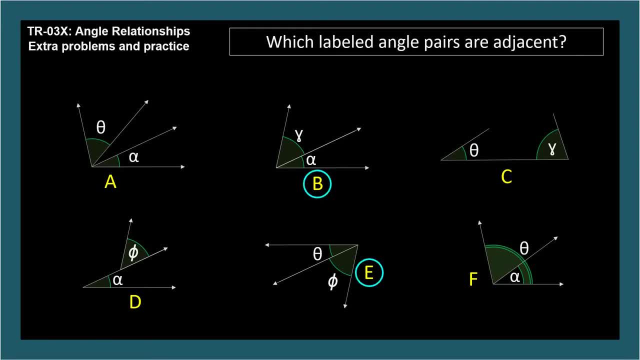 B and E. If you said F, that's understandable, but there's a subtlety that adjacent pairs are very similar. I'm going to start with the B and E: B and E. If you said F, that's understandable, but there's a subtlety that adjacent pairs are very similar. 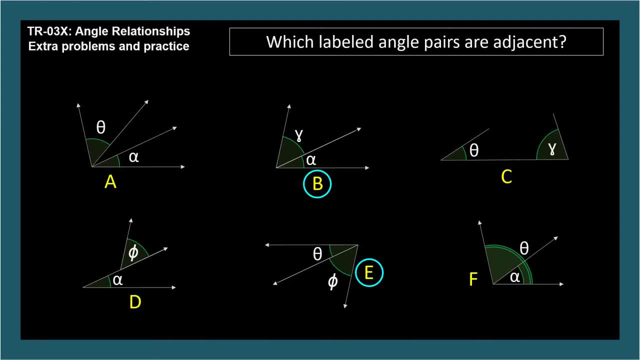 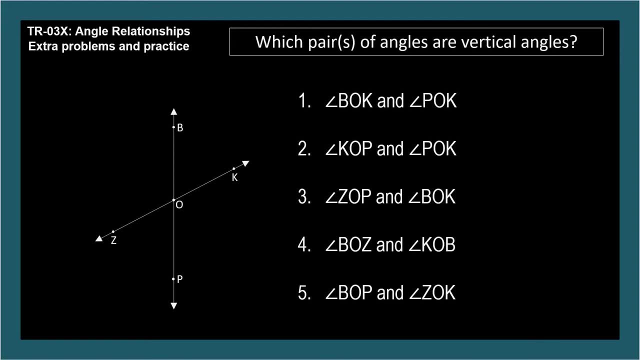 Recent angles can't be overlapping and in Diagram F, angle alpha is completely inside angle theta. Which pairs of angles are vertical angles? Angles ZOP and angle BOK are vertical angles since they're on opposite sides of the intersection. Angles ZOB and POK would be the other pair of vertical angles. 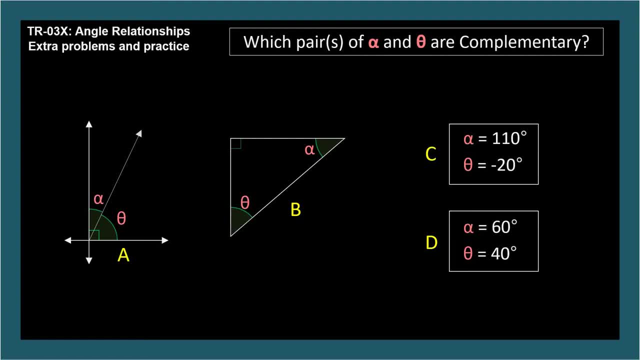 Which pairs of angles- alpha and theta- are complementary. Pause and I'll give the answer. Scenarios A and B depict complementary angles. Complementary angles are positive angles that sum to 90 degrees. Scenario C sums to 90 degrees, but they aren't both positive. 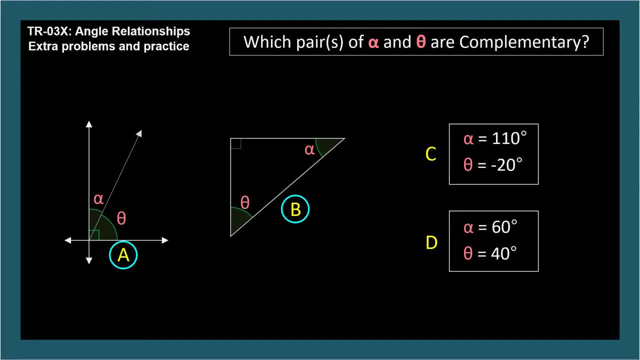 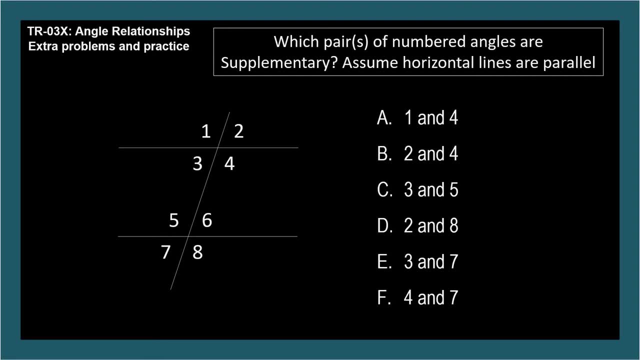 And scenario D sums to 100 degrees instead of 90.. Which pairs of numbered angles are supplementary? Assume the horizontal, The horizontal lines are parallel. There's more than one correct answer, so pause and note them and I'll give the answers all. 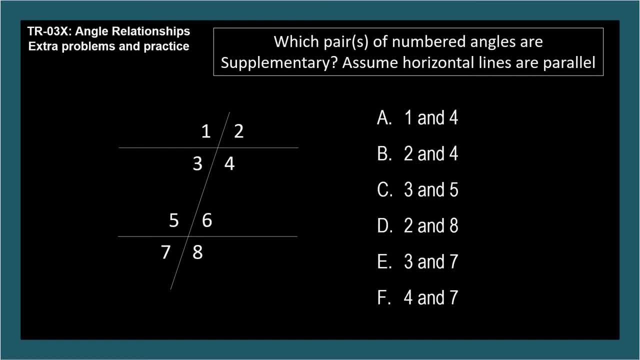 at once. B, C, D and F are supplementary. Answer F has a little twist. Angle 4 is congruent to angle 8, which is supplementary with angle 7.. So angles 4 and 7 are supplementary. What's this line called? 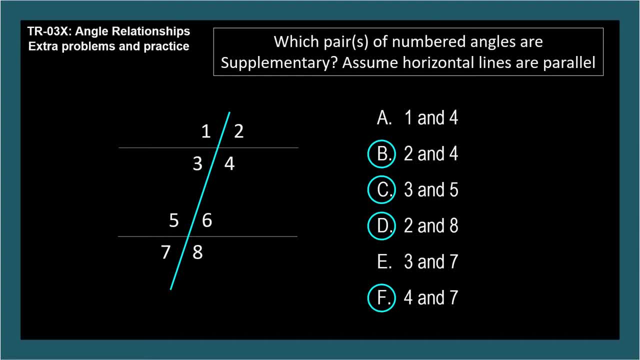 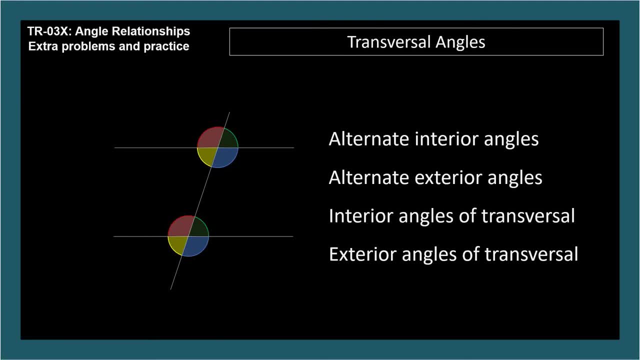 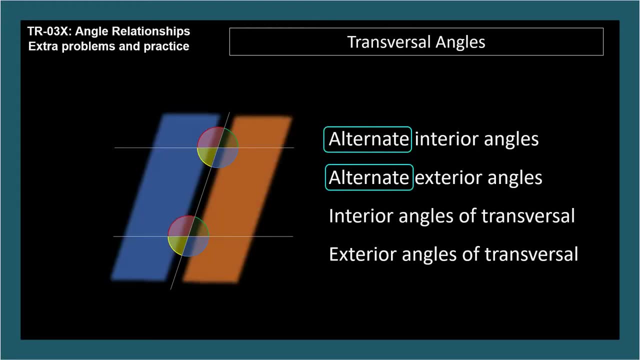 Transversal or transverse. Here are some extra helper slides for identifying transversal angles. Here are their names. They can be confusing. The word alternate means opposite side of the transversal. An alternate pair of angles would have one angle on each side of the transversal. 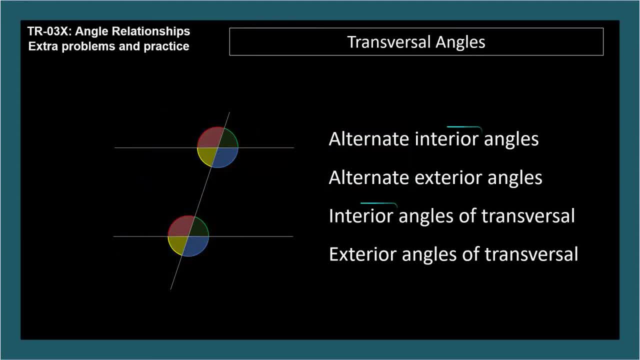 The word interior means inside or between the parallel lines. The word exterior means outside the parallel lines. The word inside means inside. Let's see lines. So alternate interior means opposite sides of the transversal and between the parallel lines. So these are alternate interior angles. and so are these Alternate interior angles are congruent. 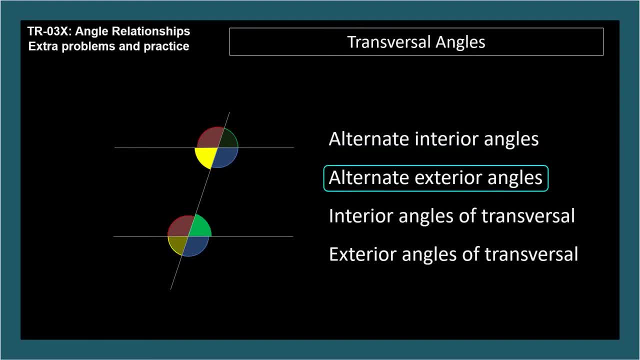 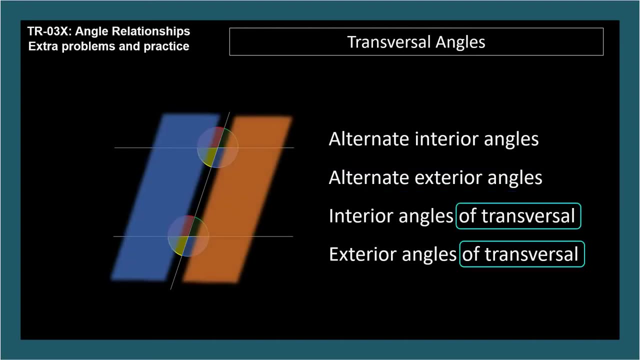 Alternate exterior angles are on opposite sides of the transversal and outside the parallel lines. So these are alternate exterior angles and so are these Alternate exterior angles. are also congruent Of transversal or of the transversal means. the angles are on the same side, not the. 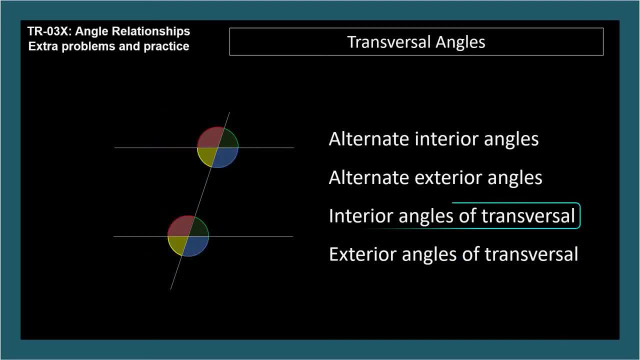 opposite side of the transversal. These are interior angles of transversal. They're between the parallel lines and on the same side of the transversal. These are also interior angles of transversal. These pairs of angles are always supplementary. Exterior angles of transversal. 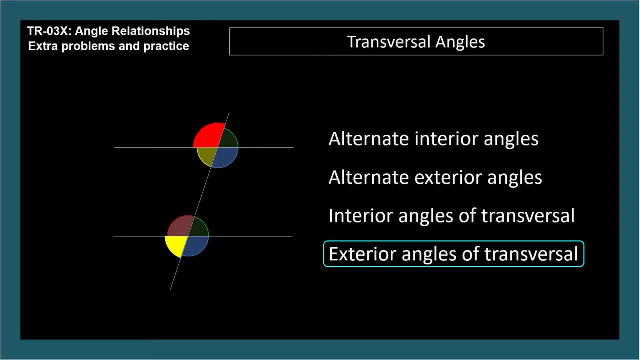 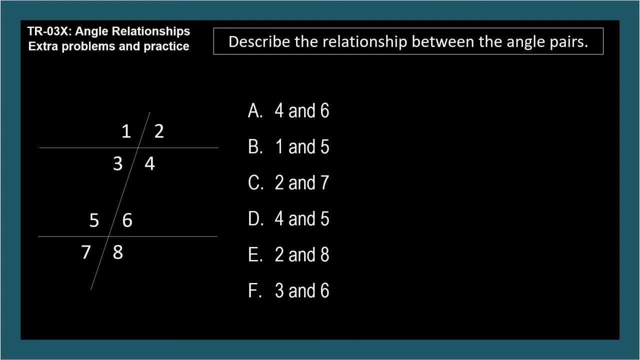 are outside the parallel lines and on the same side of the transversal. So these are exterior angles of transversal, and so are these Exterior angles of transversal are always supplementary. Describe the relationship between each angle pair. I'll go one by one. so pause as you like. 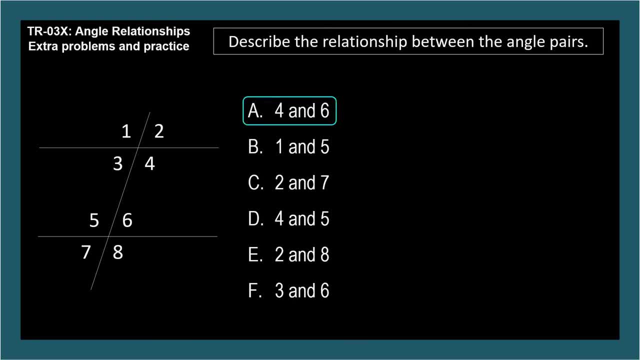 Angles 4 and 6.. They're interior angles of transversal: Angles 1 and 5.. Corresponding angles: Angles 2 and 7.. Alternate exterior angles: Angles 4 and 5.. Alternate interior. 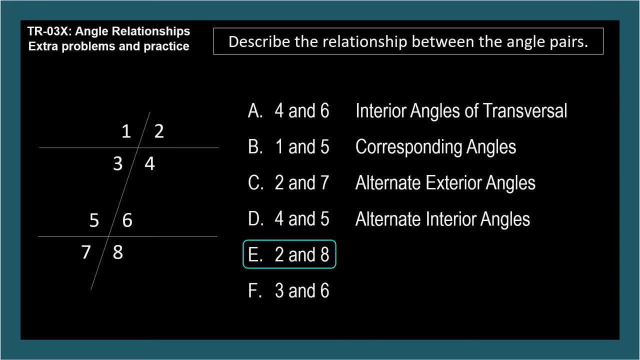 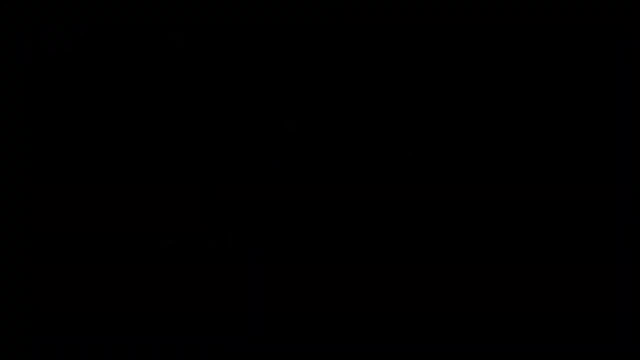 angles- Angles 2 and 8.. Exterior angles of transversal, Angles 3 and 6.. Alternate interior angles- Angles 6 and 9.. Original angles of transversal Angles 6 and 8. Agrica Lock. An analogue angle daha. Our position on uniform angles are the two Questo. It depends on the angle widely evaluated, but I like it individually with. isn't it a bit weak to to balance with too low angles, For example? it's better of the angle is higher than two angles.